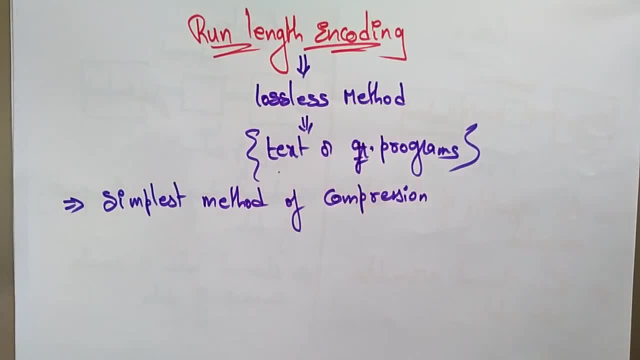 Okay, so let's see the example to understand what is this? lossless run length encoding data compression. Let me take an example. Suppose if you take an input, the input I'm taking it as A, A, A, B, B, C, D, T, D. So this is an input I'm taking. I want to compress this file. 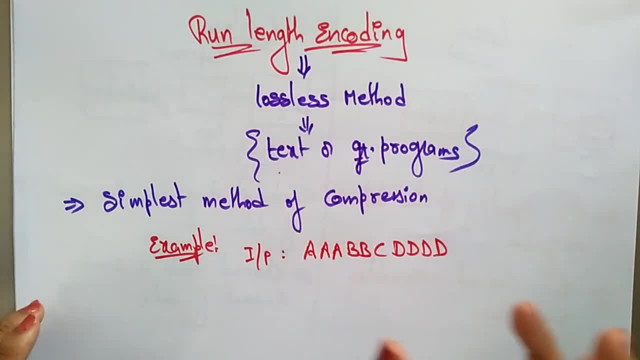 This file consisting of text or program. So this is a text, So these file I need to be compressed. So the compressed file here is, that is, we call it as encoded. The encoded file of this input is: So: instead of A, A, A, the encoded it will take 3A, Because there are three A's here, The consecutive three A's here. So that's why, instead of writing all three A's, just writing three A's. 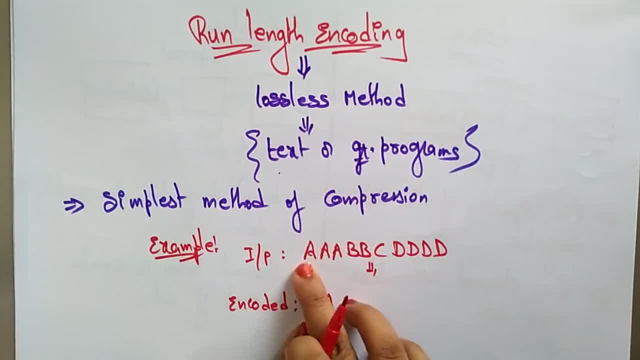 So here the file size is reduced because here three words or letters are there, But here only two letters are there. Now coming to here: BB, Okay, so BB. instead of writing every time BB, I'm just writing 2B, Okay, and C. here only one. C is there. D, D, D, 4D is there, Okay. instead of writing all the letters, you just added the numbers. So this is a compression. 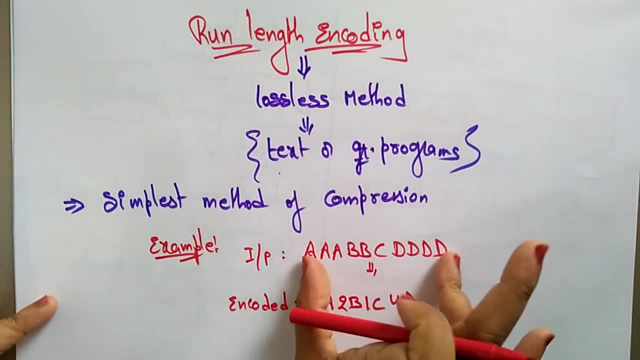 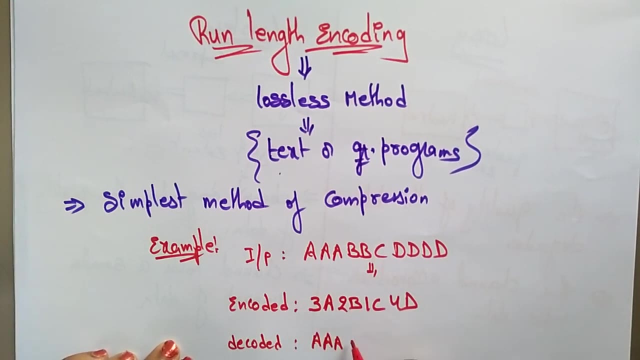 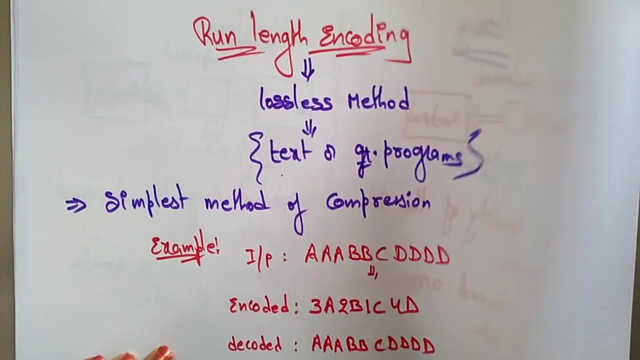 So that's why I'm saying it is the simplest method of compression. Whatever the input you are taking, that will be encoded And after, at the time of decoding the instead of 3A, it will be decoded as 3A. It replaces with A, A, A and 2B, It replaces with BB and 1C and 4D. So let me take another example to explain it clearly. 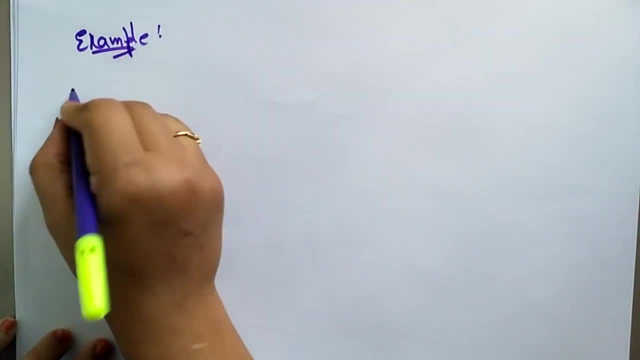 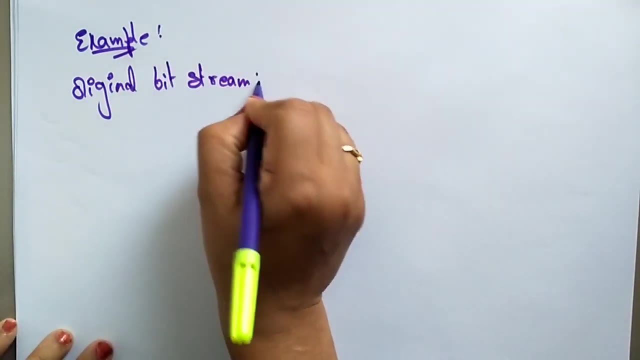 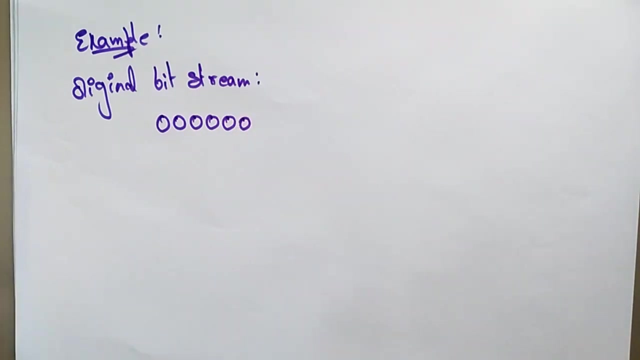 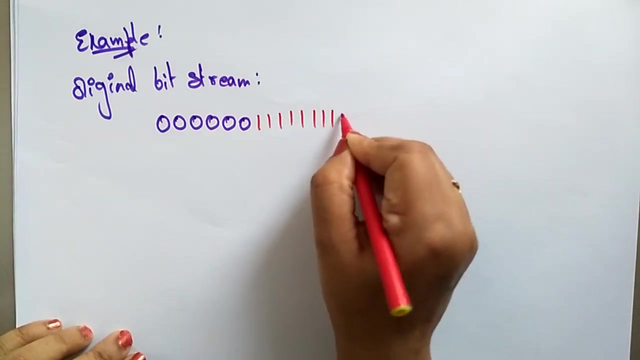 So let me take the numbers. The original bitstream is original bitstream. Let me take this bitstream First. let me take six zeros: 1,, 2,, 3,, 4,, 5, 6.. Six zeros. And let me take 14 ones: 1,, 2,, 3,, 4,, 5,, 6,, 7,, 8,, 9,, 10,, 11,, 12,, 13,, 14 ones. 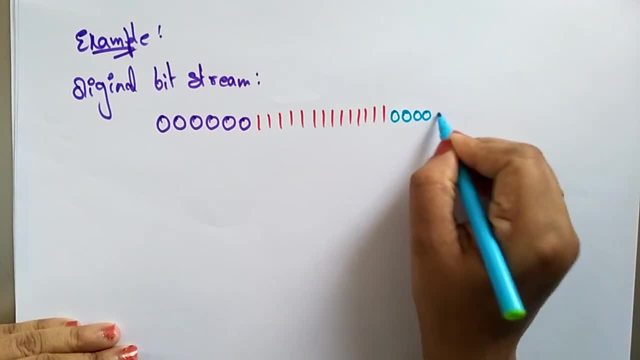 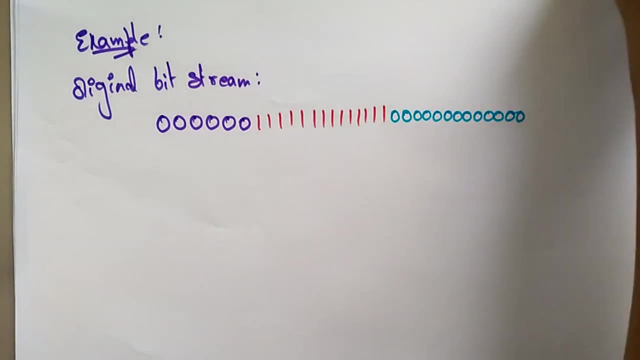 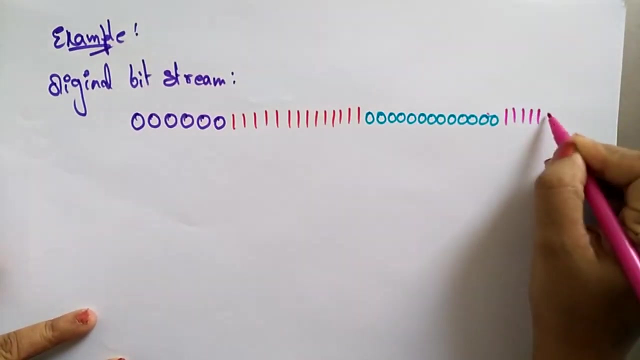 Again, 13 zeros: 1,, 2,, 3,, 4,, 5,, 6,, 7,, 8,, 9,, 10,, 11,, 12,, 13, 13 zeros, And let me take nine ones. Okay, I want to show you how this data will be compressed: 3, 4,, 5,, 6,, 7,, 8,, 9.. Okay, So this is my original bitstream. 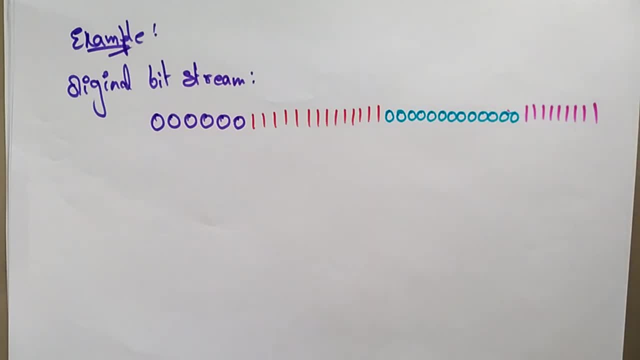 So what is the size of this bitstream? The total: here six zeros are there And here 14.. 1 bits are there, and here 13, 0 bits are there, and again here the 9, 1 bits are there. so the total: 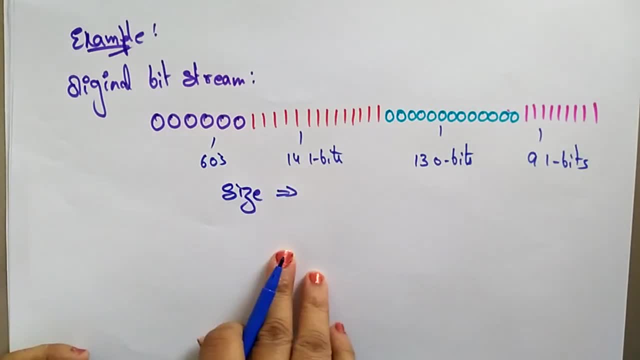 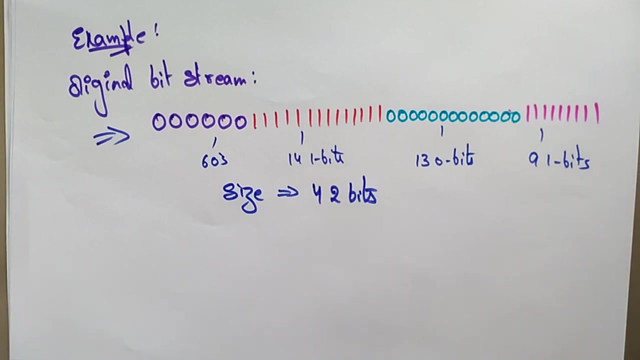 size of this bit stream is starting before compression. the size of this bit stream is 42 bits. the total size of this bit is: it's a 42 bits. okay, now i am compressing by using the run length encoding. how i am compressing by using the run length encoding. now let's see the first step. 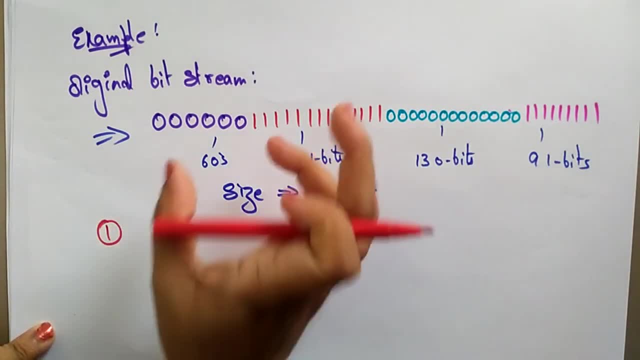 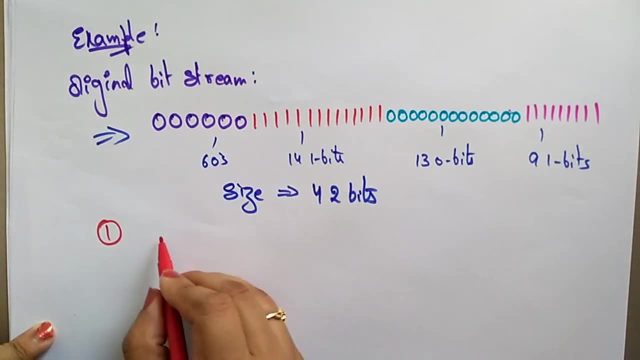 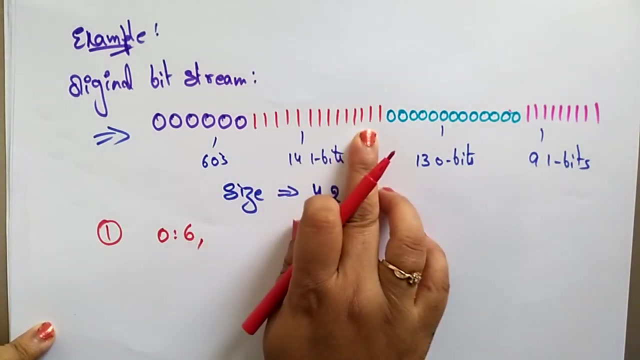 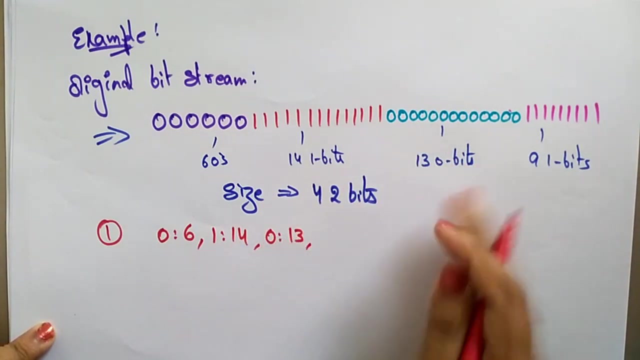 step one in the run length encoding. so whatever the redundant data is there so that you have to be reduced. so instead of writing six zeros, i'm just writing zero appear at six times comma, and here the one, 14 ones are there, and again the zero, 13 zeros are. 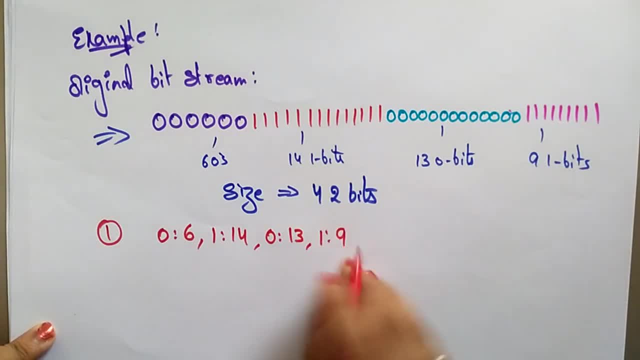 there and again one nine ones are there. so this is the compressed one. so now, finally, the resulting. the second step, the resulting five bit byte is bytes, is so zero. what is six represent in the form of ones and zeros, so that the system can understand. that is a decoding, the machine language. 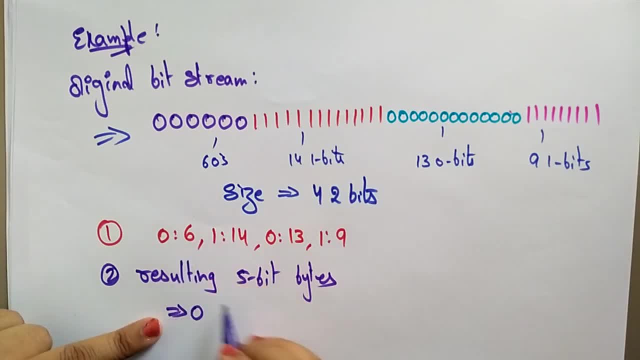 can understand, it's only in the form of ones and zeros. so six is nothing but zero, one one zero, zero. one, one zero is nothing but a six. so this completely, it is a five bit byte. okay, now one is there 14. the 14 can be represented as: